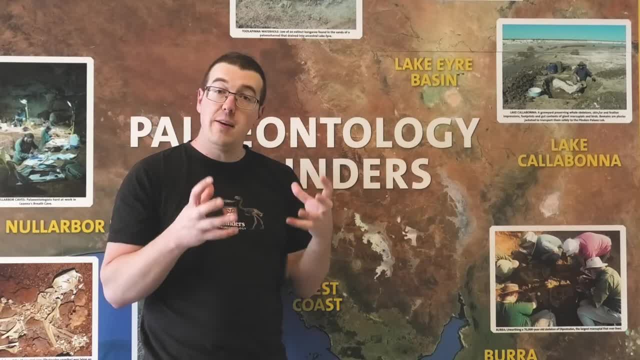 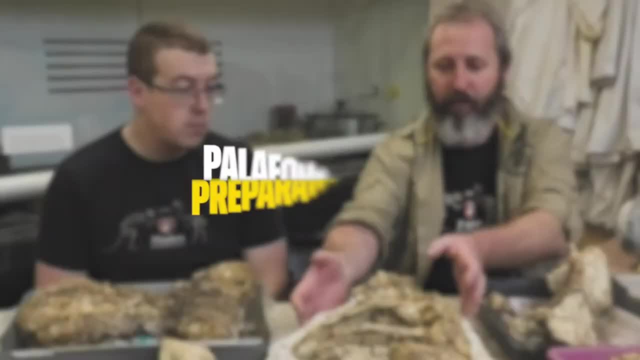 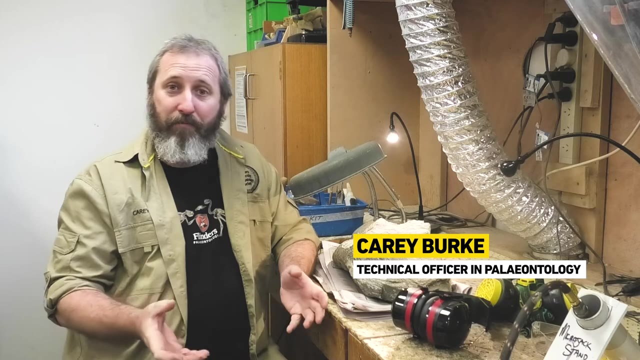 all of the fossil study takes place, So you'll be hearing from various different Flinders paleontologists about what they're studying and what they're doing. G'day, my name's Kerry and I am the lab technician here at Flinders University in the paleontology. 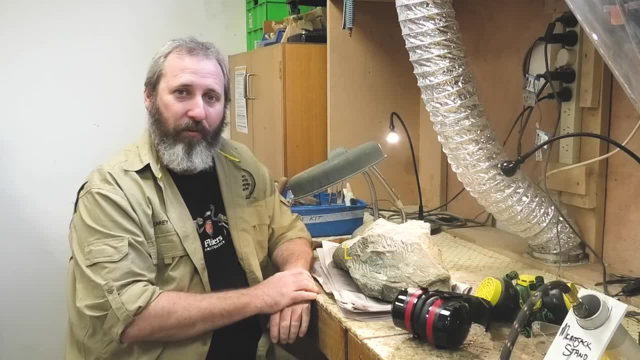 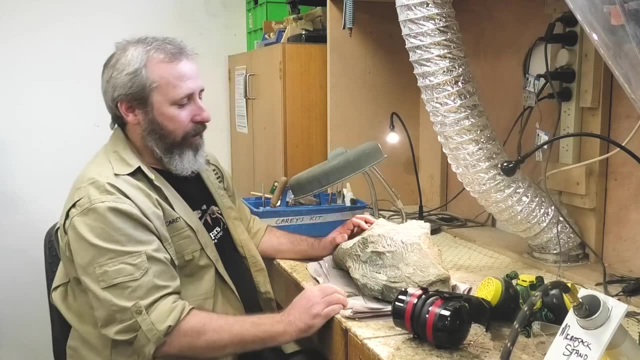 department. So in paleontology I would be more known as a preparator, because fossils need to be prepared for study. So I'm going to be talking to you about the preparation of the fossils. So I'm going to be talking about the preparation of the study. So one of the ways that we prepare fossils- 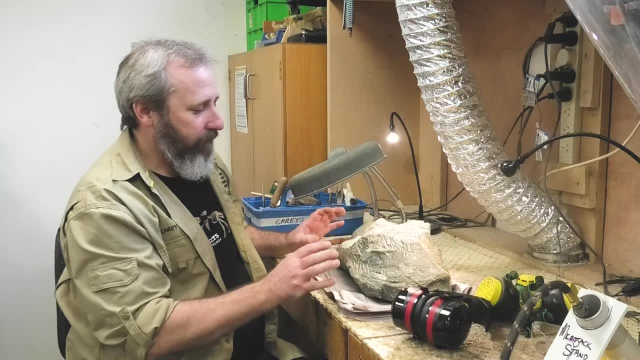 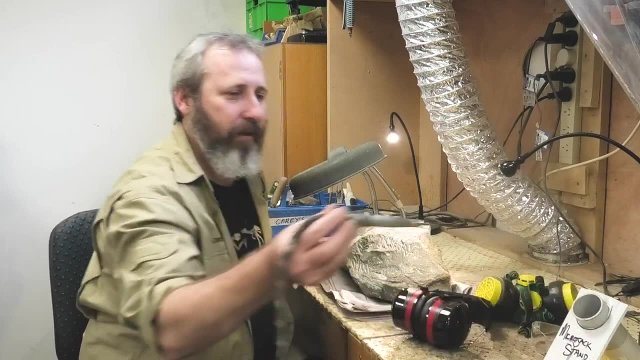 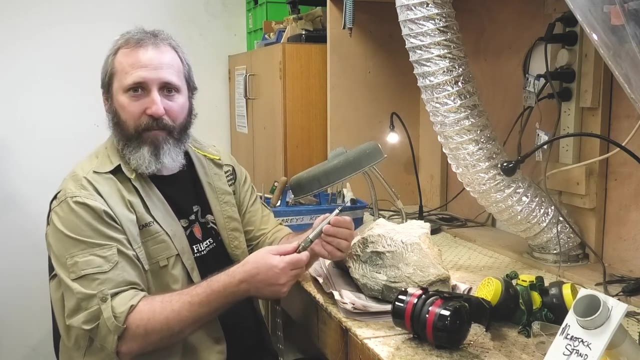 is, of course, to release them from their rock, what we call the matrix. Now, some fossils are particularly hard, difficult to remove, so we've got some special tools. This is called a micro jack. This is basically a tiny, tiny jackhammer. It's an air powered tool. the 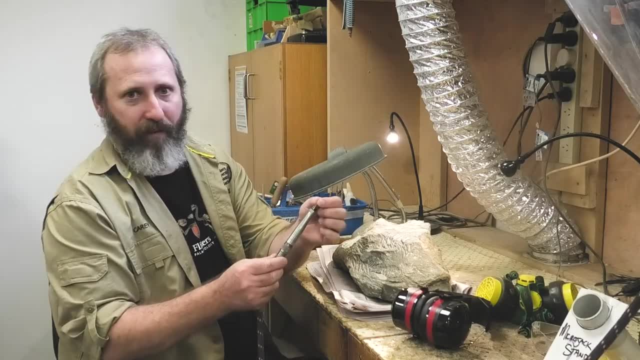 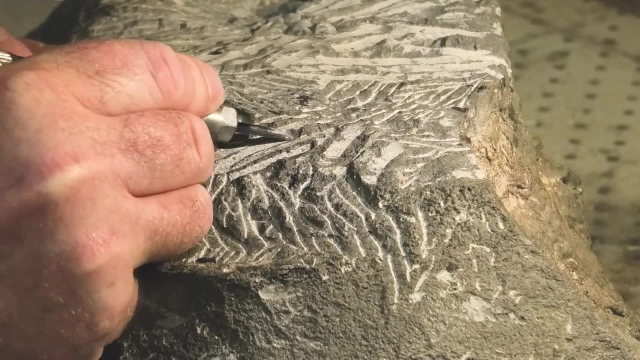 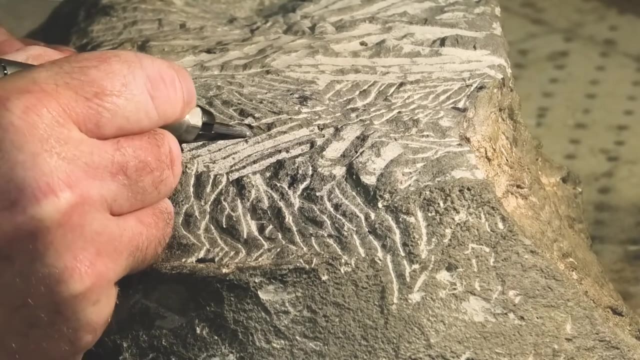 little blade at the end oscillates up and down a hundred times per minute. you just use this to chip away at the rock extremely carefully and release the bone. Micro jacks come in many different sizes, from extremely large to tiny ones that I use under a microscope. but for a specimen like this, this size here is: 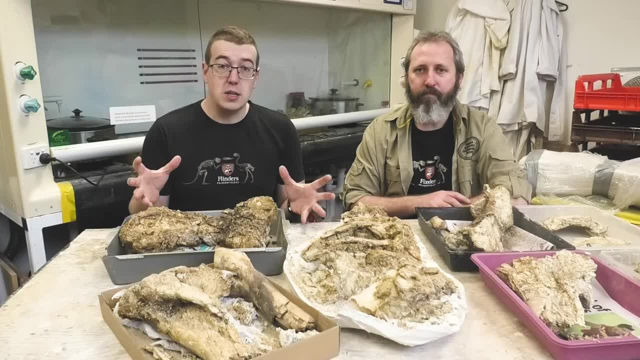 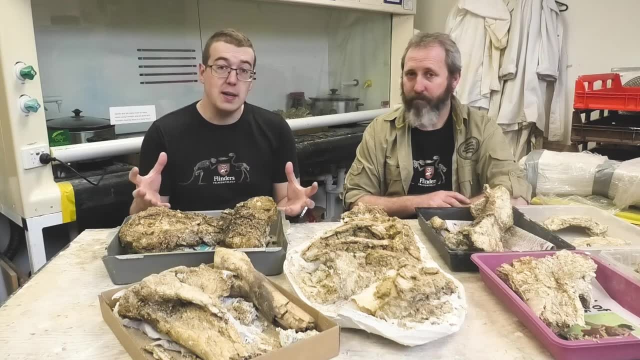 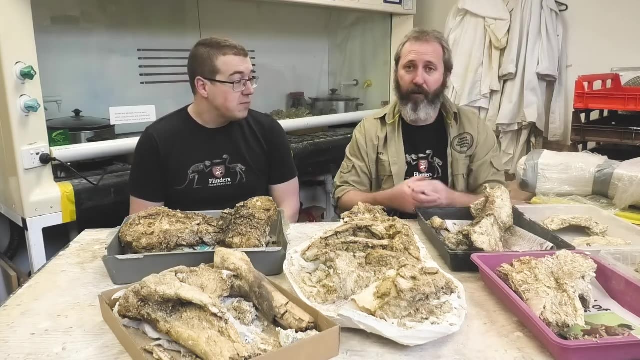 ideal. So here we've got a collection of bones that have actually been found out at Lake Calabona, and Kerry's going to tell us a little bit about how we go about collecting these bones and some of the challenges that are faced when we collect these things. Okay, well, the first thing to know about the Lake Calabona- 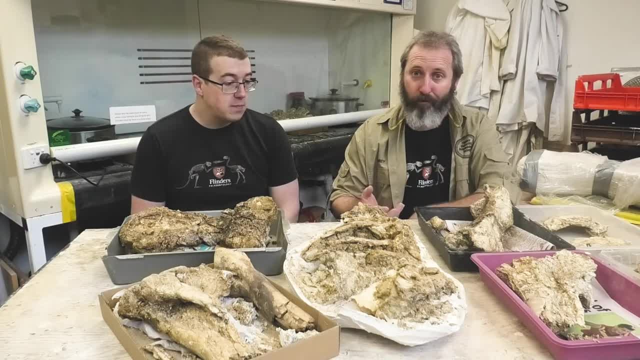 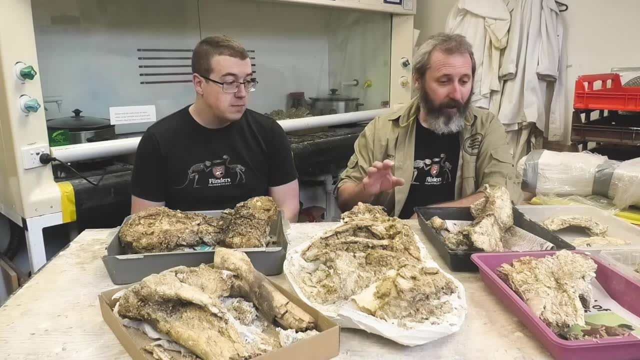 specimens is that Lake Calabona is an extremely remote location. It is a long way from home to go and get these guys and there's nobody else out there to help you. The second thing about Lake Calabona is it's a salt lake. It's muddy. 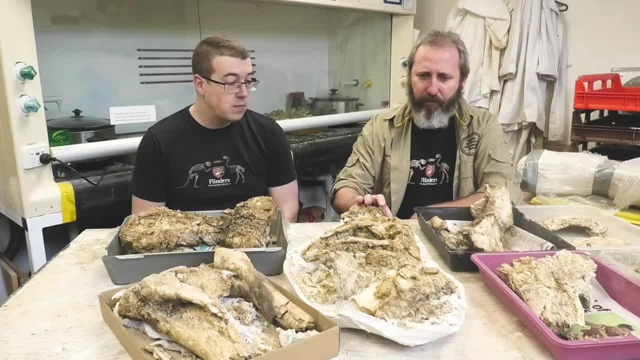 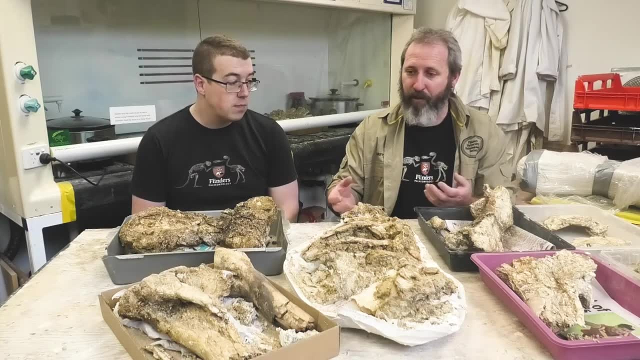 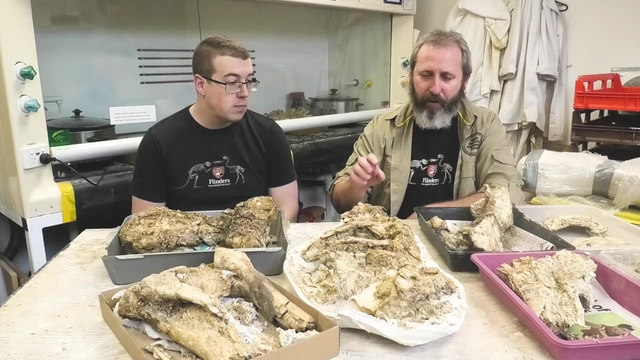 it's salty. The fossils are preserved in this environment and as soon as you begin to excavate them, they can begin to deteriorate because you've changed what preserved them in the first place. So to collect a fossil, we would walk around the lake until we found the tiniest bit. 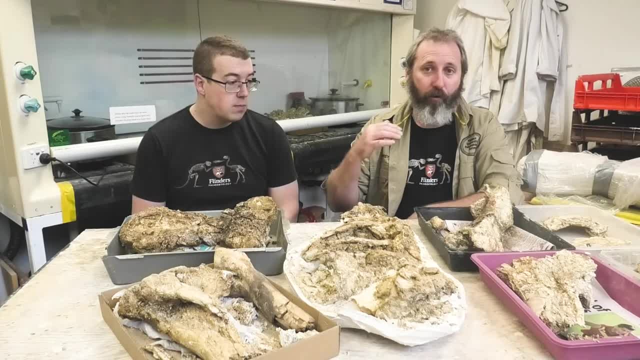 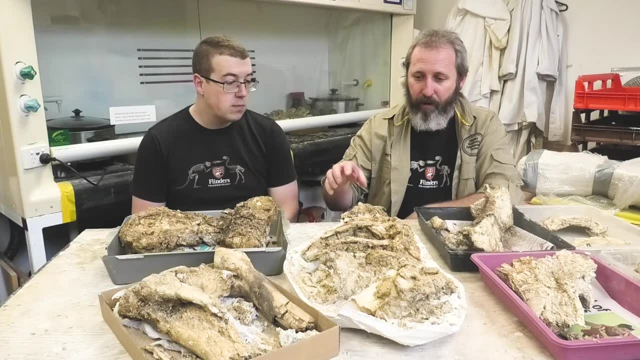 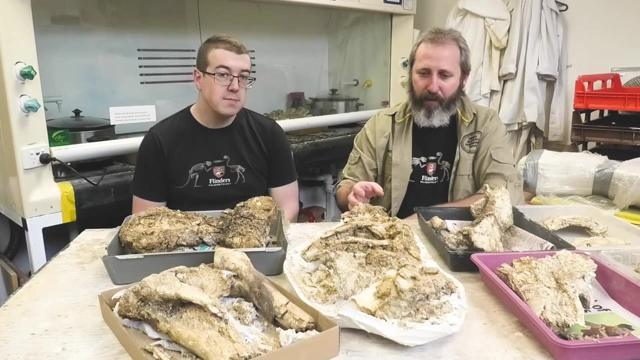 of bone sticking up over the surface of the lake. Erosion would naturally expose these fossils. Then we dig a huge trench around the bones, We wrap a plaster jacket around them until we make almost like a white egg to protect them, and then those eggs come back in the car with us all the way back. 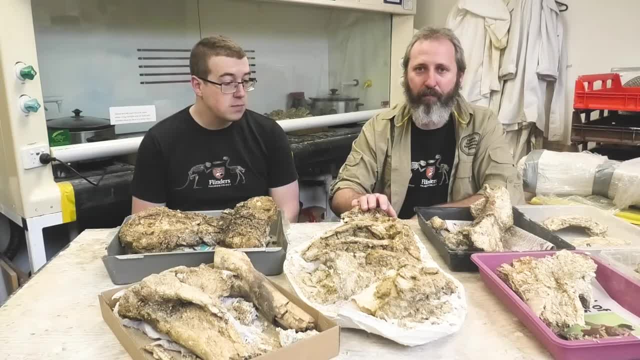 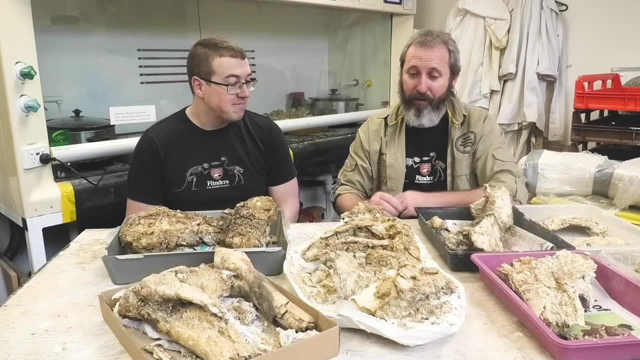 to the lab, and in the lab we open them up and we actually see what we've got with our fossils. But the fun doesn't end there, does it? No, like I said, you've changed the preservational environment. so as soon as you open your eggs, these 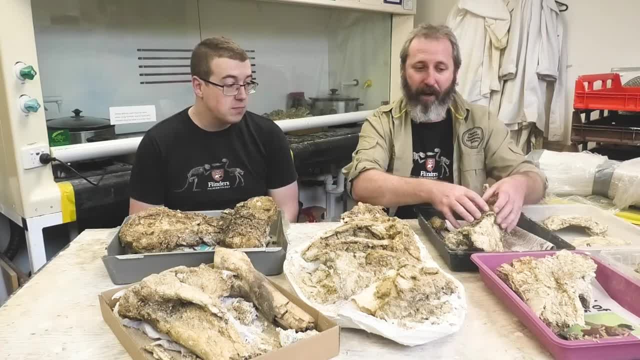 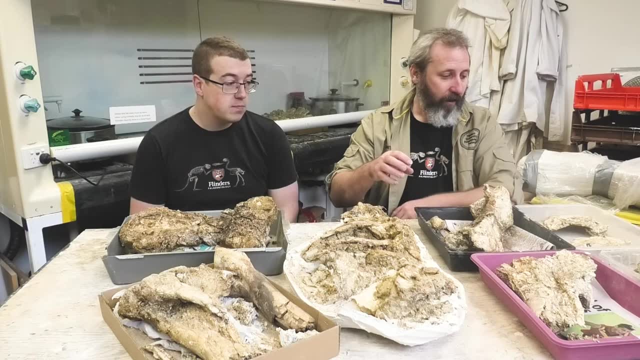 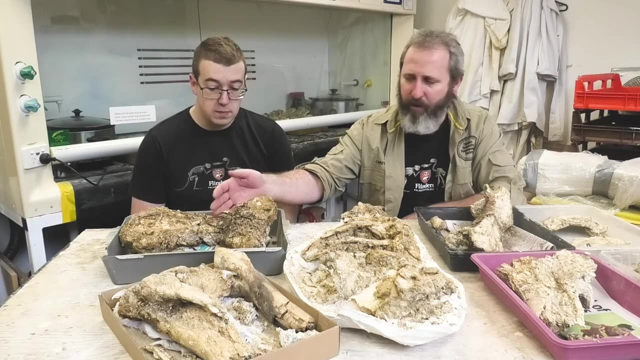 fossils start to degrade, Salt can come out of the bones, form a nice little salty crust on them and actually deteriorate and smash the bones up. And a lot of these bones are not preserved perfectly, As we can see here. this one's crushed and smashed through weight of sediment on it, through all sorts of 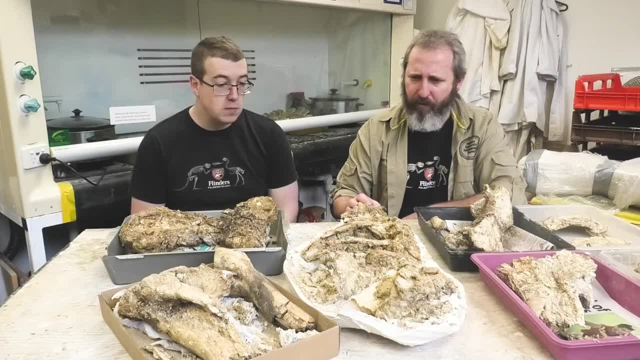 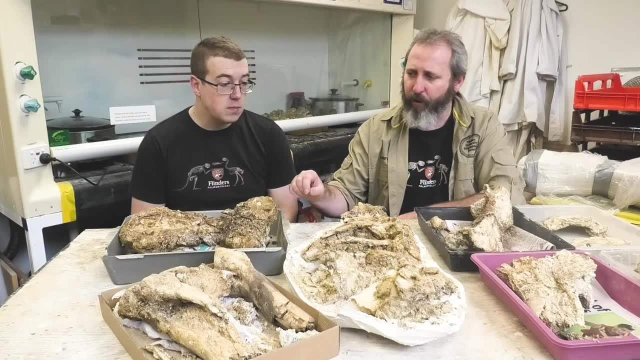 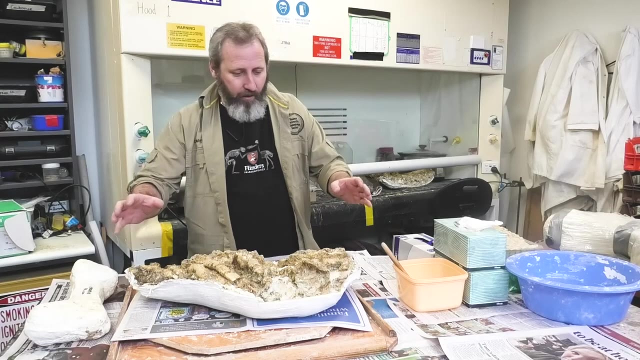 erosional factors, and it's been well over 40,000 years. A lot can happen in that time to a specimen. So my job here is to not repair these bones, but to make sure they never come apart in the first place Today. plaster jackets- I've got a. 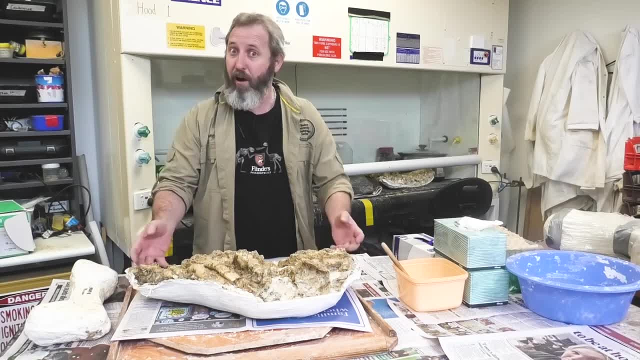 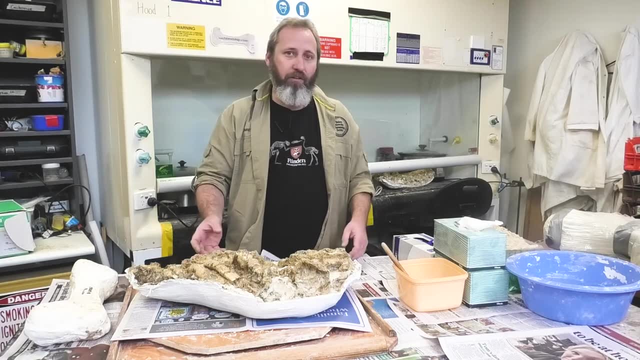 my fossil here. This has come out of the field. It's been half prepared. The other half underneath still needs a lot of work. Plaster has been used in this industry almost for the entire length of the industry. It's a great, cheap, portable. 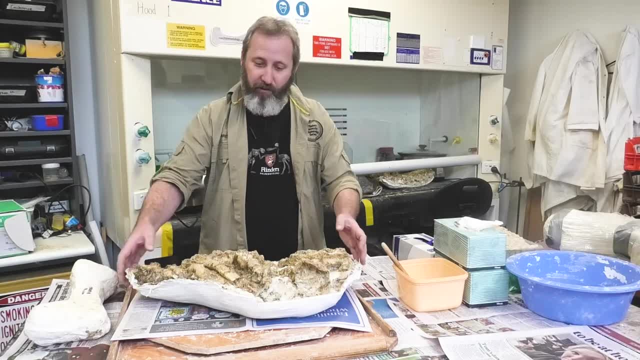 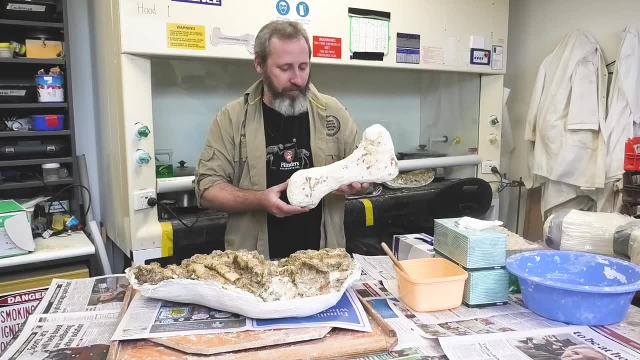 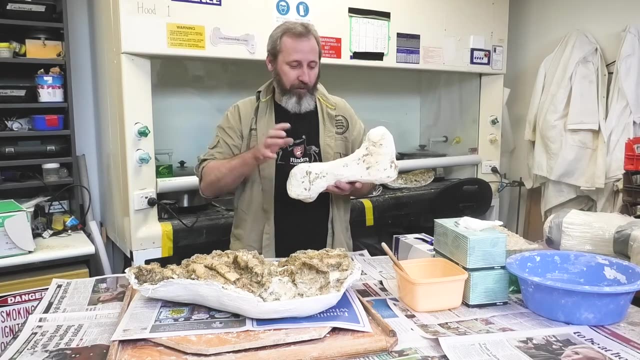 substance that can make hard shells around, otherwise impossible to move fossil material. So you may have seen something like this come out of the field when people are digging fossils. This is just a plaster jacket wrapped around the shape of a bone. The plaster jacket means that we can pick. 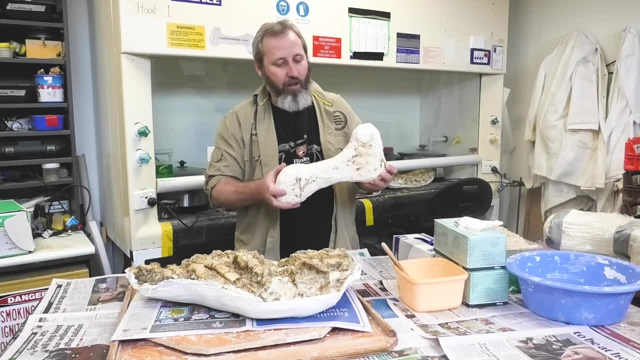 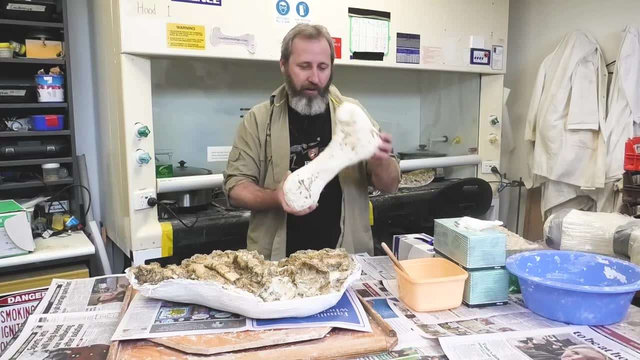 this up. It's tough. We can transport it. If this bone wasn't in this plaster jacket, I would not be able to pick this up. It would crumble into hundreds of tiny little pieces. So this keeps bones safe until we can get them back into the. 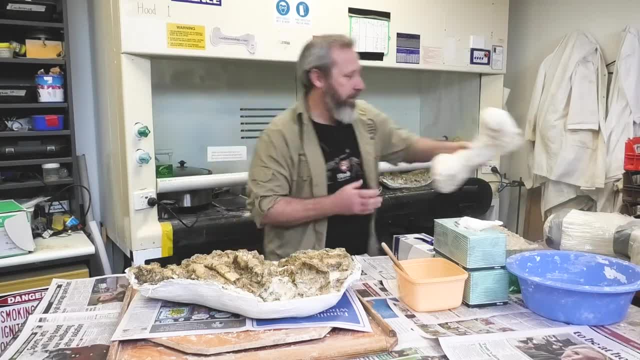 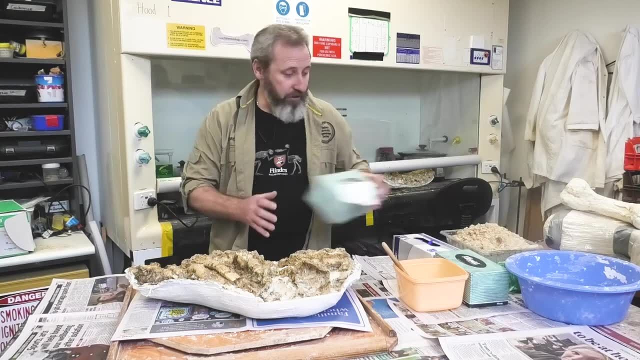 lab, harden them, clean them, get them ready for study. The process of plaster jacketing is very simple. First of all, we use tissues and some water. I'll stipple them on with a brush to get a nice form-fit layer. This will be. 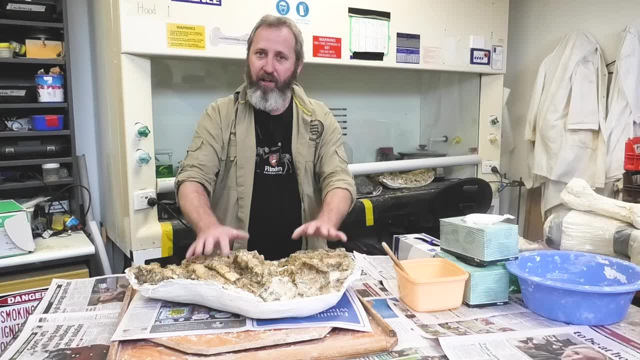 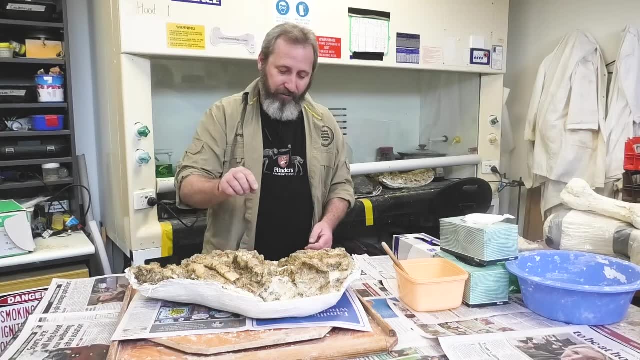 our separating layer between our precious fossil and the subsequent layers of plaster that we'll put on. The separating layer means that as I'm digging down again, I know exactly where to find that fossil, because there'll be a coating of tissue and nothing else will stick to the fossil itself After. 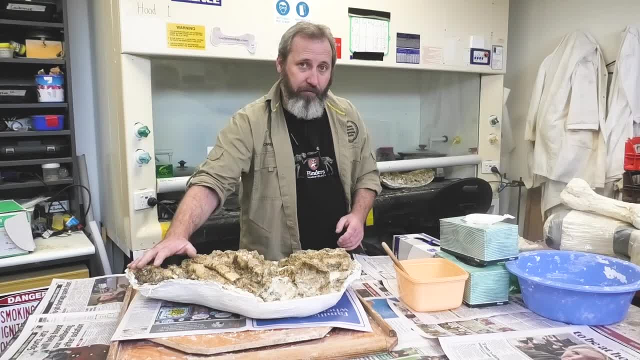 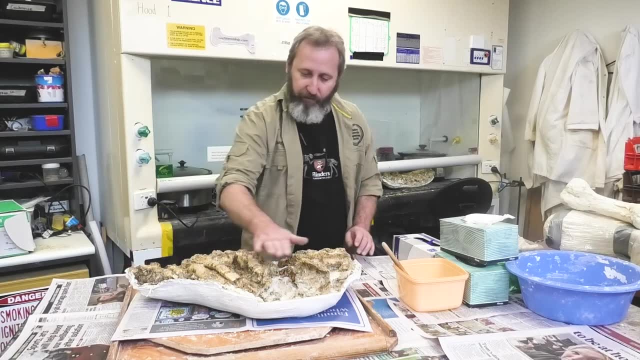 that I'm going to put a layer of wet sand over the top of the fossil and the sand is going to fill up all of these holes, all of these gaps, all of the little details, and make a nice smooth dome for me to put my plaster shell over. 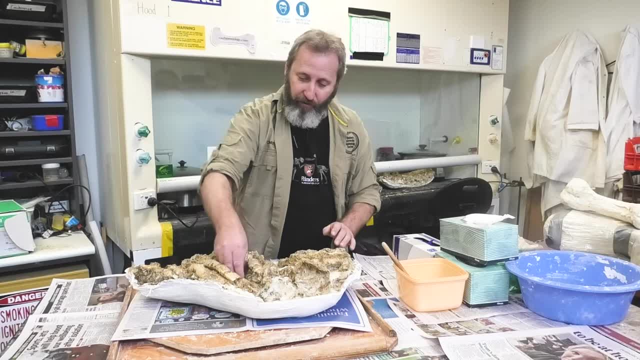 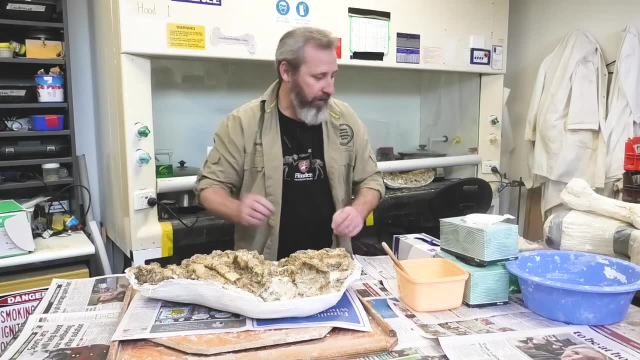 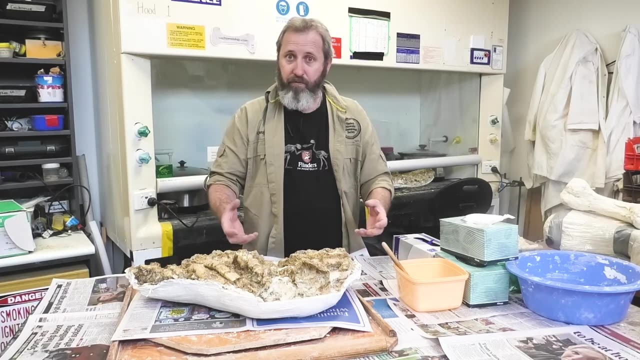 If I don't have a nice, smooth dome, the plaster itself will go into these crevices and will catch on the fossil and we can actually break fossils trying to get the plaster off again. And the last step will be, of course, the plaster jacket itself. Often we will use hessian and powdered plaster in the field. 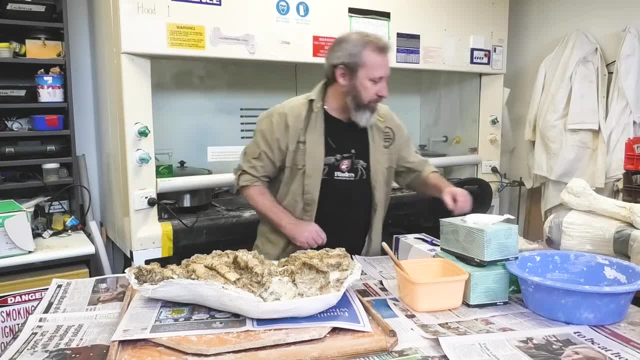 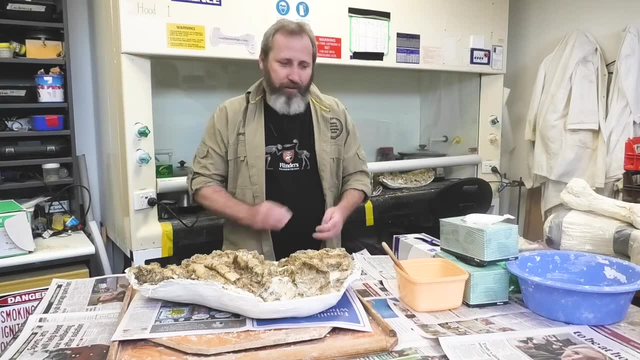 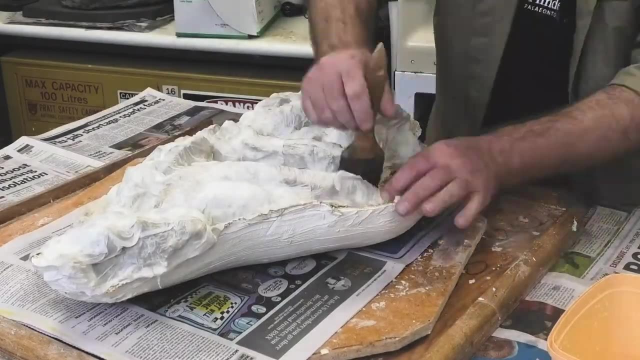 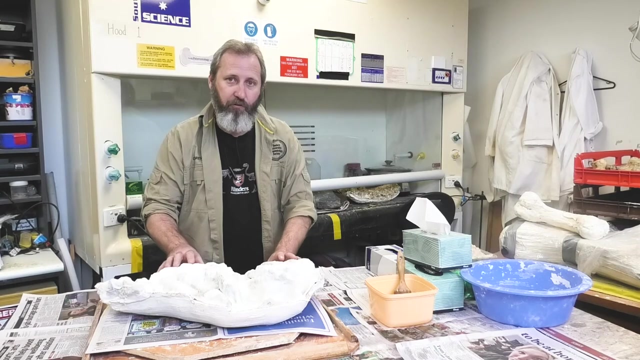 because it makes a nice strong, thick, heavy jacket. But today, because we're in the lab, I'm going to use these pre-made plaster bandages. Let's get on with it. I've finished stippling tissue all over the fossil. It's a nice separating layer. 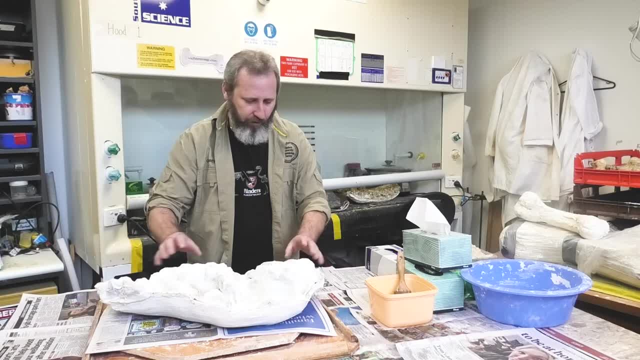 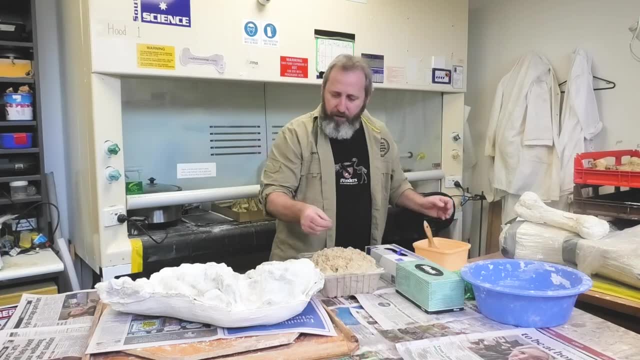 probably about two layers thick of tissues just to keep it all safe and secure. Now I can put this away. bring out some nice, slightly wet sand and I'm going to coat this with a protective layer of sand. Remember when I turn this upside down. 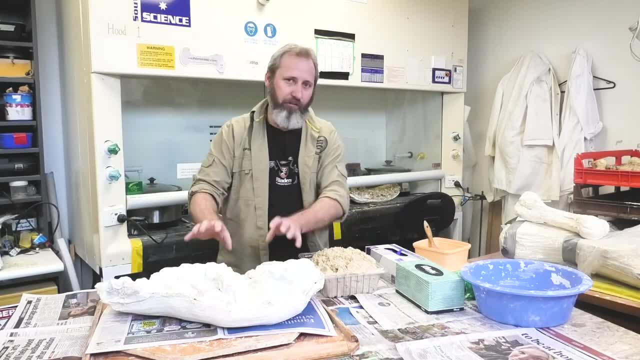 this fossil will rest in this sand. The sand is the cushion that's going to keep this from snapping off all of these delicate little pieces. I've finished my sand. as you can see, I've made a little wheelsaw. it's a bit harder than you would think to cut with a drill, but part, and I think I have established that there's still room in the scever between the paper and the 못. 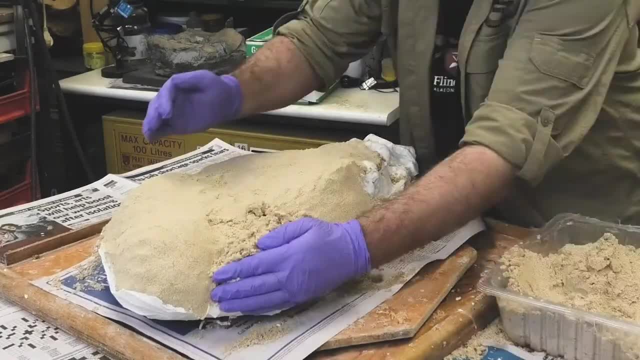 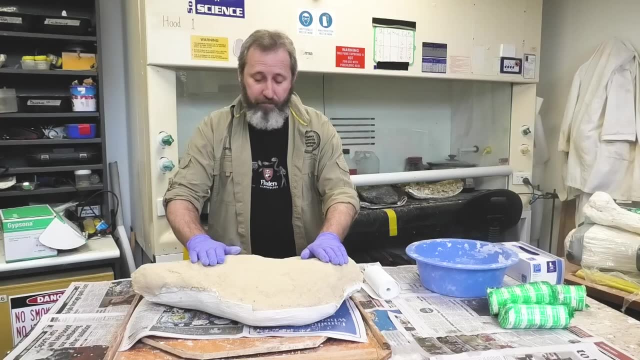 I've finished my sand. As you can see, the top layer should never get loose, at least on natural times. I've토 make just a couple ofח sand. as you can see, I've made a nice smooth shape. there's no undercuts. 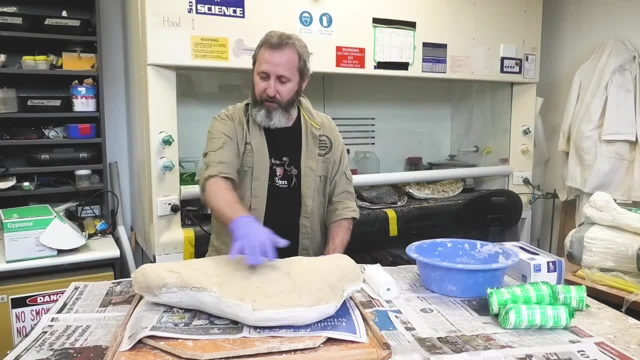 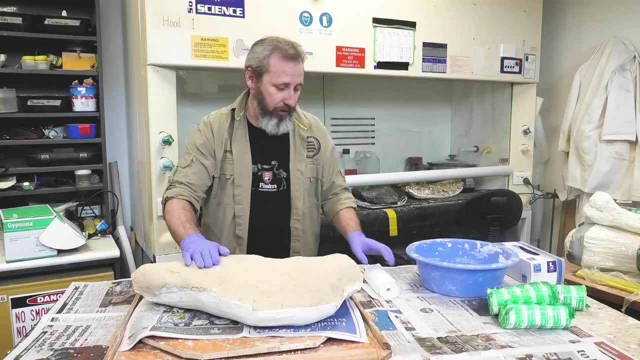 there's no places for the plaster to get caught. later on, when I need to release this fossil from here, it'll be just a matter of sweeping the sand out of all those crevices and cracks. so now I can get on with the plaster. so these plaster. 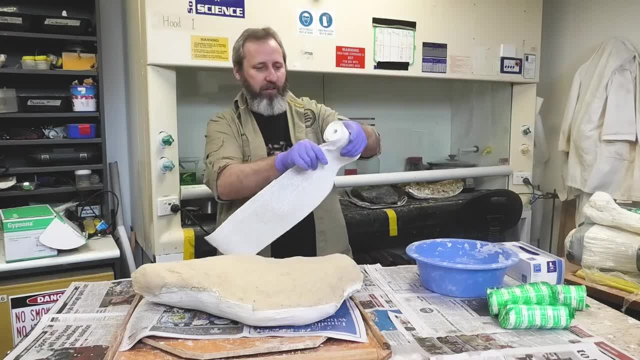 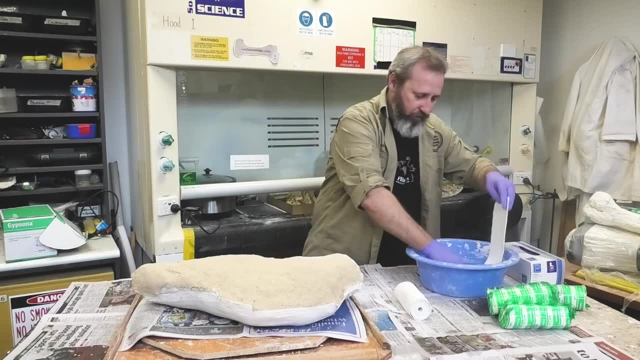 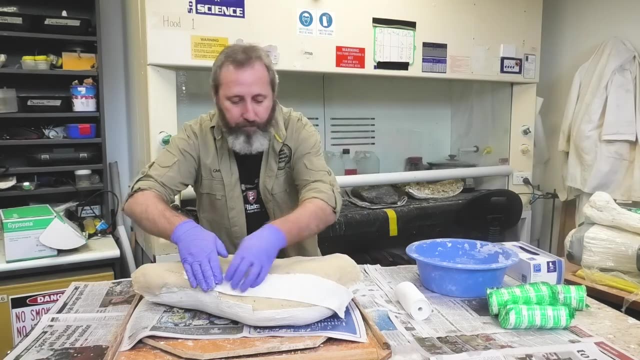 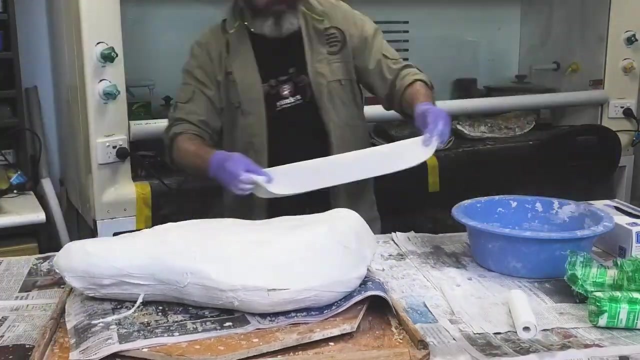 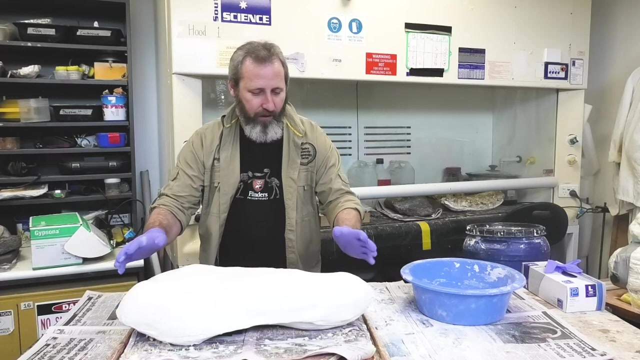 bandages are magnificent. they've already got plaster inside them. they're very, very quick and simple to use. we just dip them in some water and start to lay them over our specimen. I've got one layer of plaster bandages on this fossil now. this looks lovely and 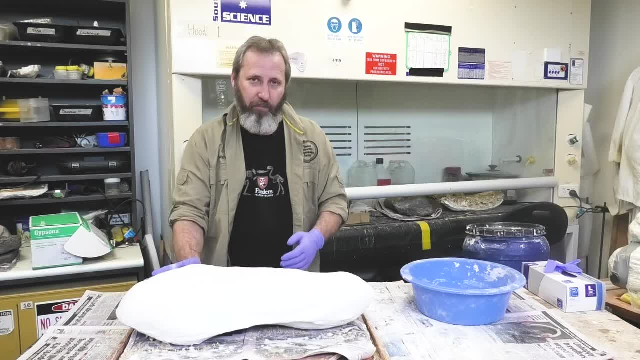 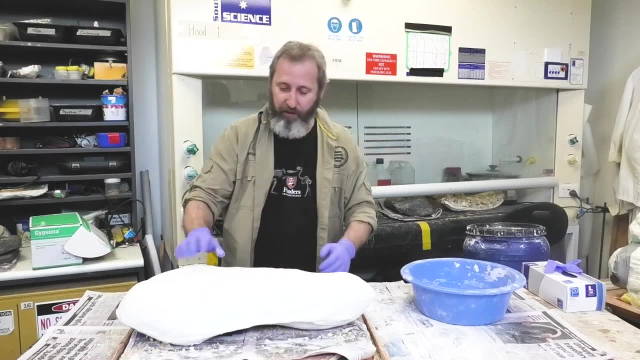 strong, but it actually isn't. this is a paper-thin coat of plaster and I'm going to take a little bit of water and I'm going to coat it in the field. we would cross strap and we would build a very, very strong, maybe a centimeter or more thick plaster block to go on this. but in the 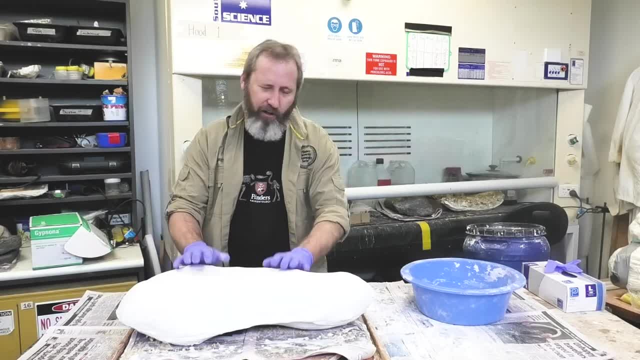 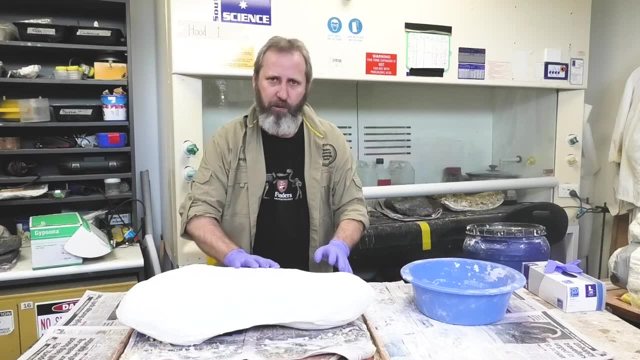 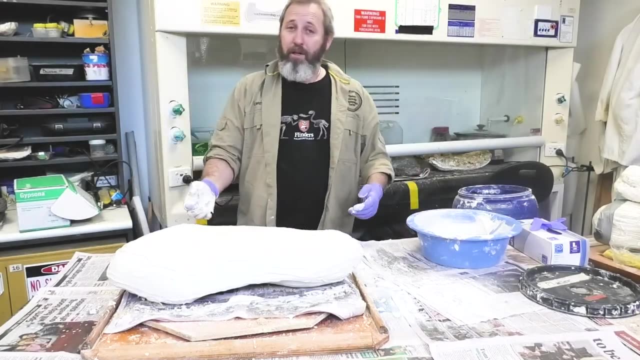 lab, because I'm just going to turn this over and remove more weight. I don't need anything near as strong, however, I am going to mix up another batch of just pure plaster and thicken this up to give it a bit more strength. easy, so what I've? 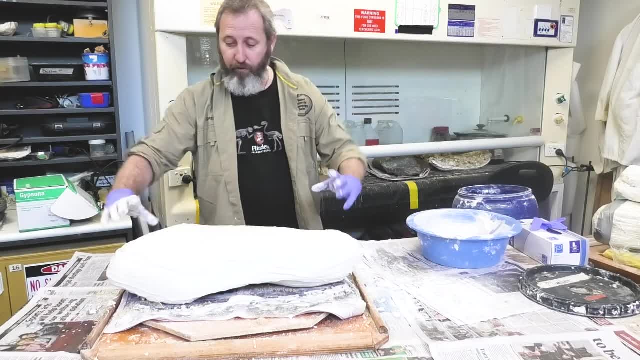 done. here is made a little bit of plaster and then I'm going to coat it with plaster and then I'll go to the other side to get that piece of plaster done. so I've got the plaster here and I'll take a little bit of plaster on this. 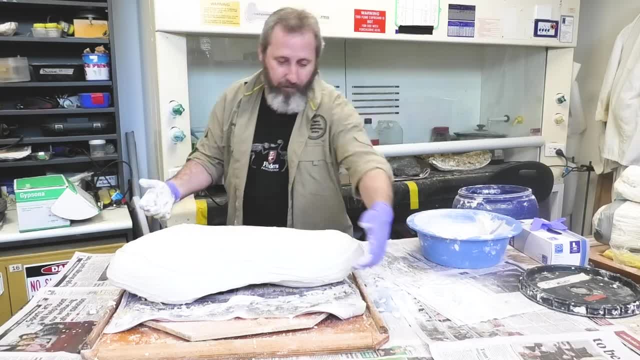 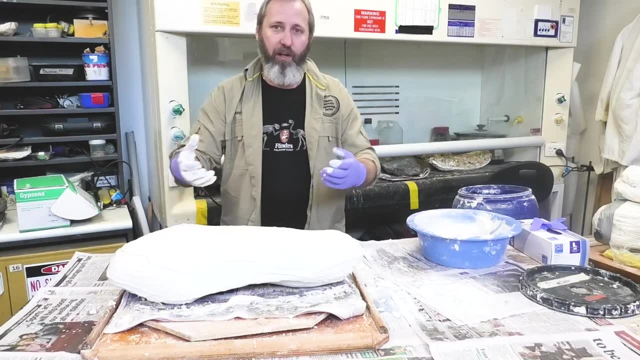 one here is made a nice solid base for this fossil to rest on. when this is finally dry, I'm going to turn it over 180 degrees then cut what's now at the bottom off of the fossil so I can access the other side without having to lift. 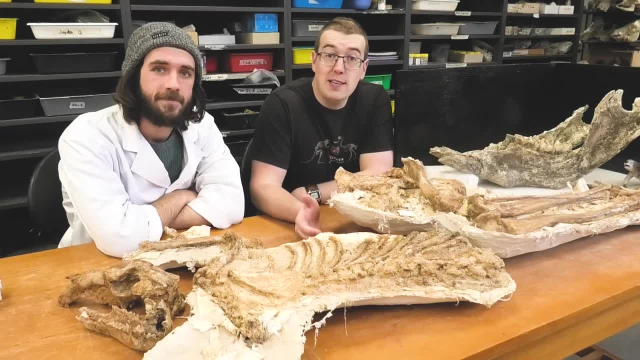 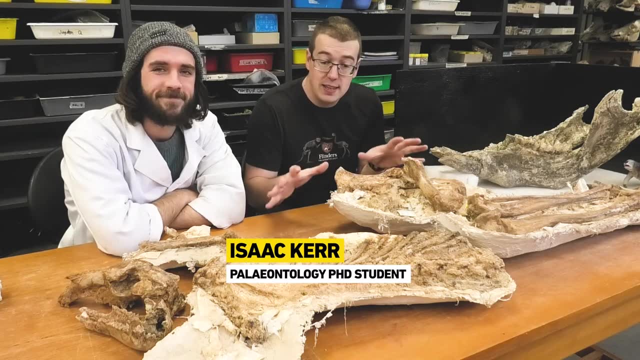 manipulate or otherwise damage a fragile specimen. this will be ready tomorrow. so here we are with Isaac Kerr. he's one of the PhD students here at the Flinders University paleontology lab and he's working on some of his problems with plaster- plaster of these fantastic fossils that are coming out of Lake Calabona. Isaac, would you like to tell us a? 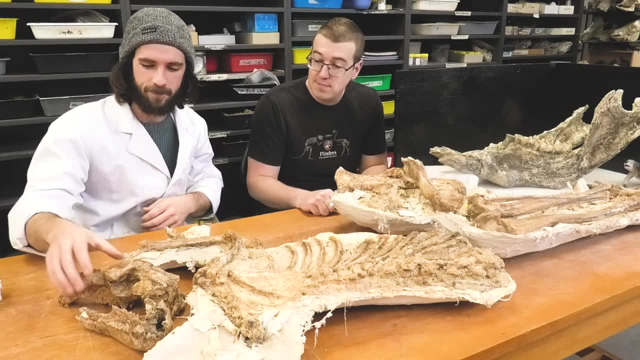 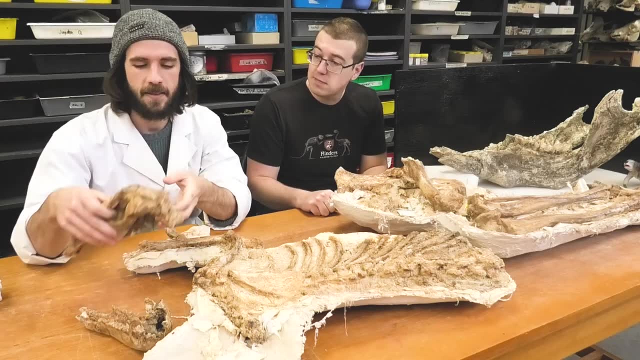 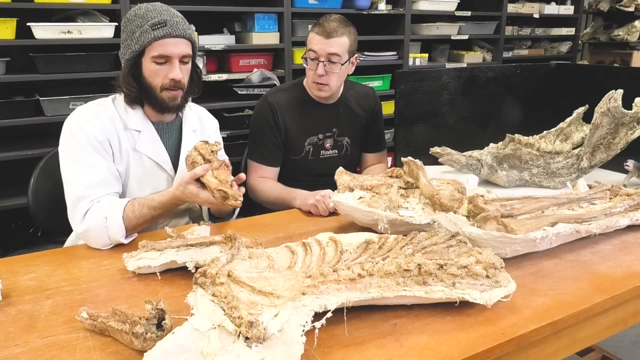 bit more about what you're working on for your PhD. Yeah, sure, so I'm working on protemnodon kangaroos, which is a genus of giant kangaroo that died out about 40,000 years ago and the very last of those we can see at Lake Calabona. This is one of them here. this is a old female protemnodon. 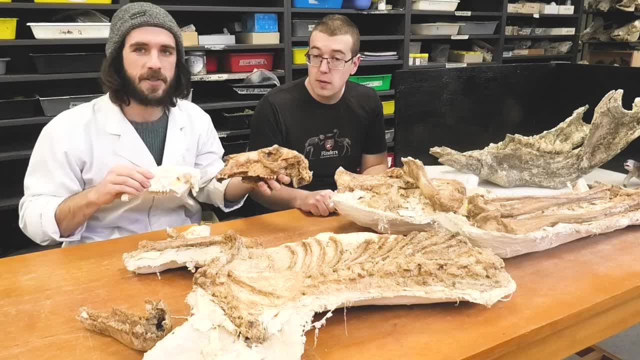 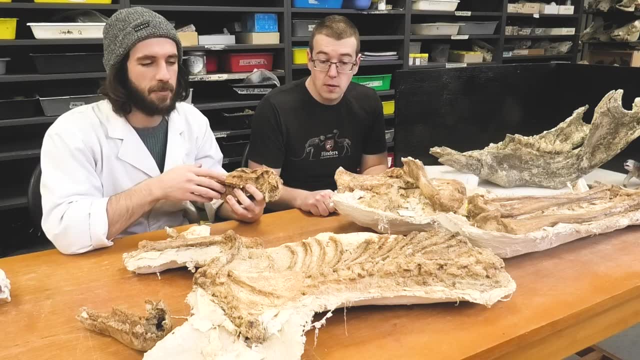 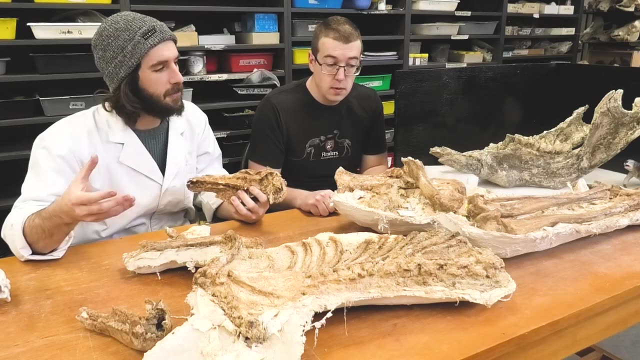 and, as you can see, when I compare it to a red kangaroo skull, there's a very, very big kangaroo and we found her lying on her side in Lake Calabona. so, unlike a lot of the other specimens, she wasn't found to have died bogged. she was lying on her side, which suggests a different. 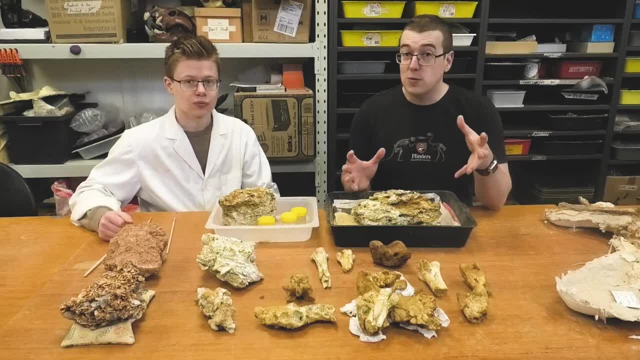 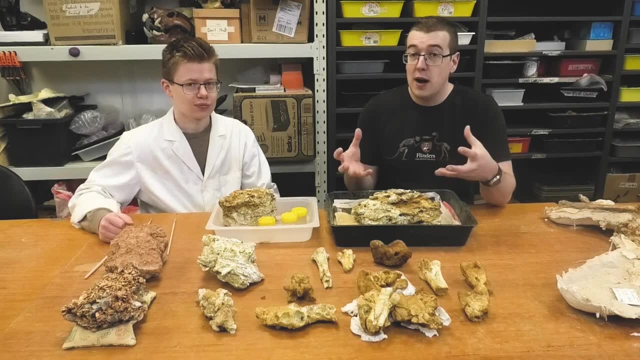 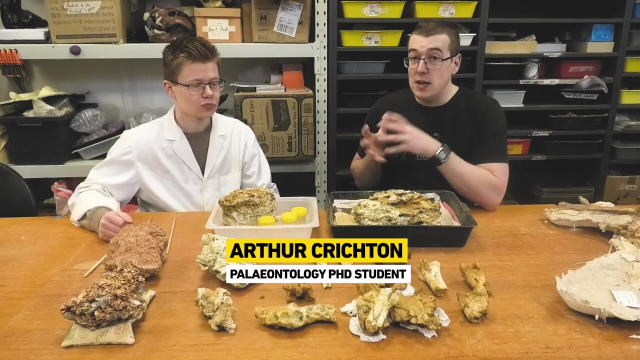 mode of death, which is very interesting. Now, not all fossils are entombed in mud. sometimes they're entombed in much harder things, and that means we need to use different kinds of preparation techniques to be able to access the fossils. Arthur Crichton is doing his PhD on one. 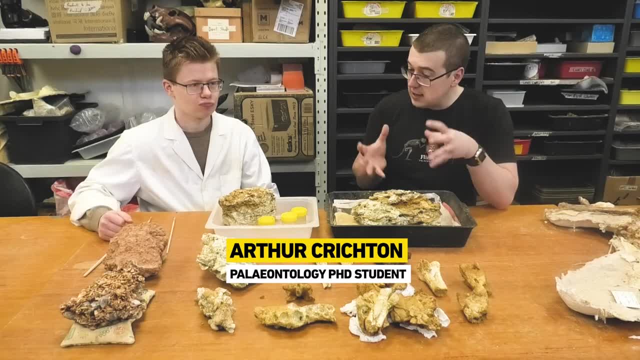 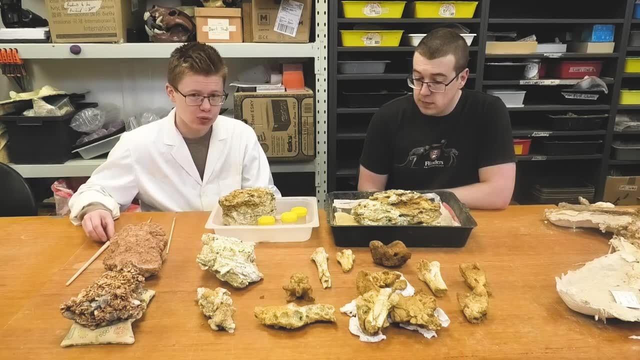 of these sites. that's quite challenging to prepare. Arthur, do you want to tell us about how you prepare these fossils? I'm doing my PhD on a site in the Northern Territory which preserves some of the earliest representatives of modern Australian marsupials and one of the 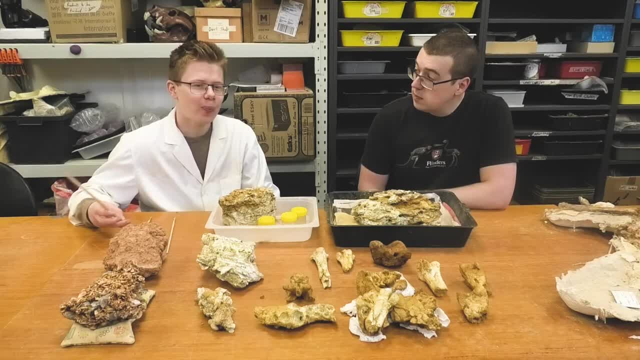 which is great, which is really exciting, is the preparation of the fossils. So I'm doing my PhD on the site in the Northern Territory which preserves some of the earliest representatives of modern Australian marsupials and one of the which is great, which is really exciting. but actually prepping out the material from the rock is really. 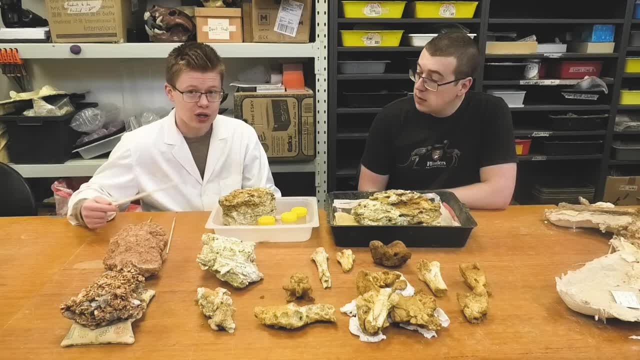 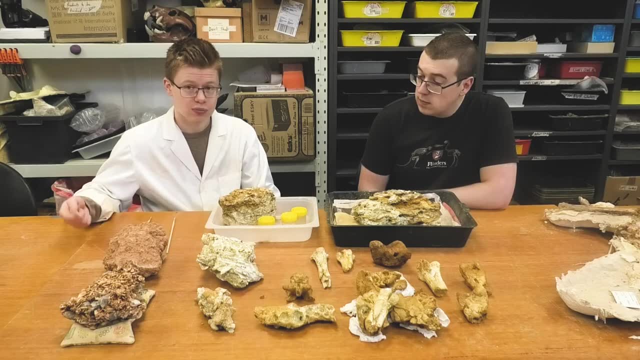 quite challenging because the material is highly fragmentary and it's relatively soft compared to the limestone which it's encased in. So I use weak acetic acid to dissolve away the limestone and extract the bones. How do you make sure that you're preserving the bone and not dissolving it? 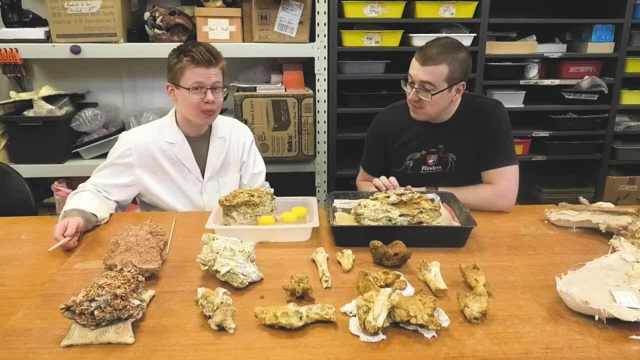 and you're preserving the bone and not dissolving it when you're doing this. So I'm doing my PhD on a site in the Northern Territory which preserves some of the earliest representatives of modern Australian marsupials and one of the and you put it in the acid. I make sure that I harden the bone every time the rock comes out of. 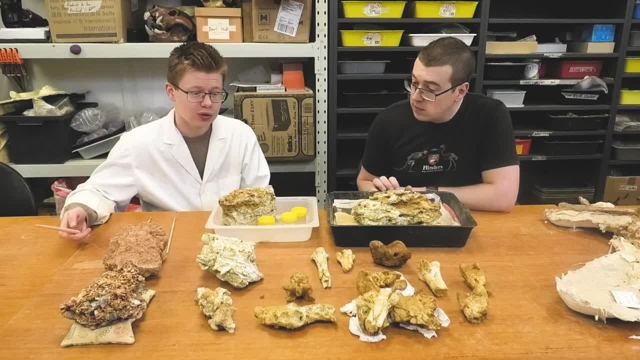 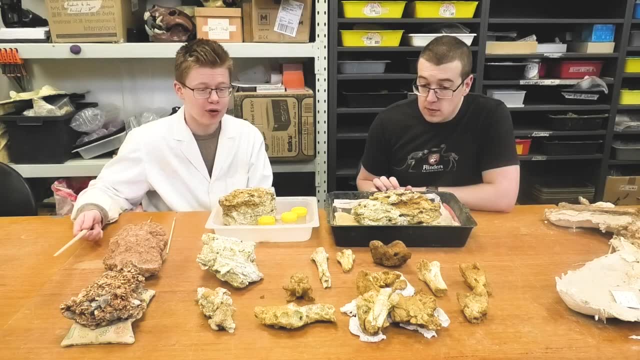 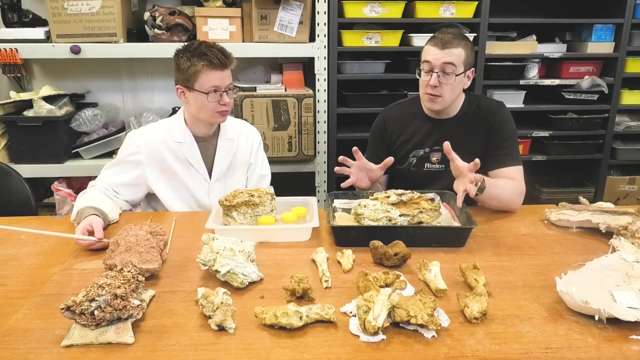 acid so that the newly exposed surfaces don't fall apart. So, for instance, this crocodile snout here took about five months to repair out. So a lot of work goes into this before we can actually see what fossils are hidden in these rocks, but they're super important. Other deposits like